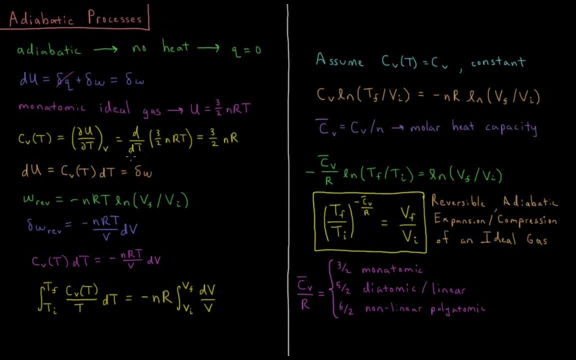 a function of T and the number of particles. but we're not interested in that right now. so U being only a function of T here, we can make that a normal derivative DDT of three-halves nRT for du dt. so the derivative of three-halves nRT with respect to T is just three-halves nR. so our heat. 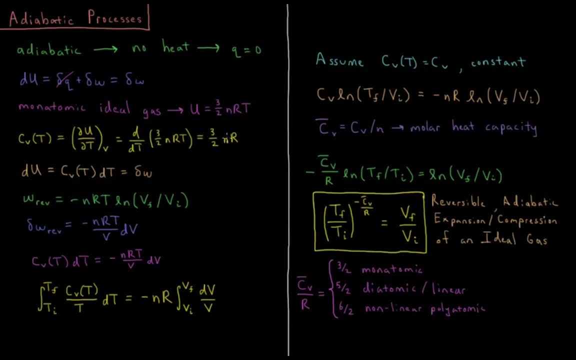 capacity for our monatomic ideal gas is three-halves number of moles times the gas constant. so the change in energy that occurs during some process is going to be du dt times DT, so the partial derivative of internal energy with respect to temperature times the change in the temperature for both. for some. 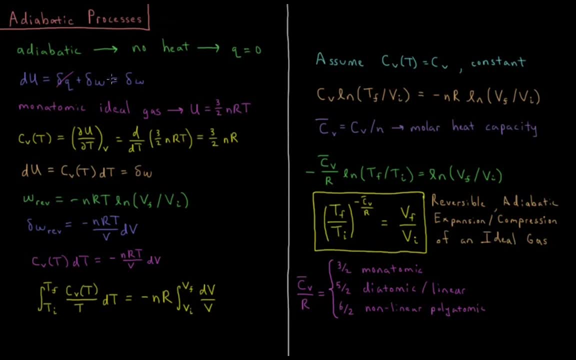 small, infinitesimal change which we defined up here, is equal to the work which gets done during that very tiny change. okay, so the reverse work that occurs during the expansion or compression of an ideal gas is equal to negative nRT. log V: final over V: initial number of moles of gas gas. 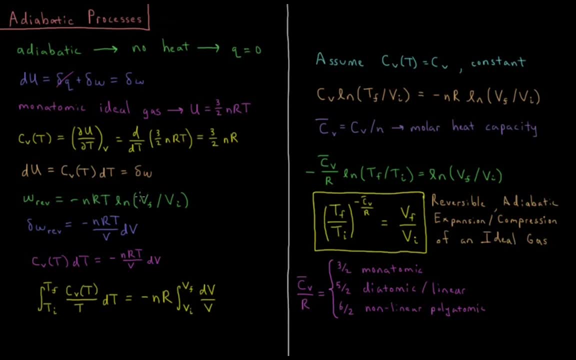 constant temperature, final volume of the gas and initial volume of the gas. so if we take the part, we take the infinitesimal of this, we get that the reversible work, the infinitesimal of reversible work, is equal to negative nRT over V dV. the derivative of log of V with respect to V is 1 over V. so 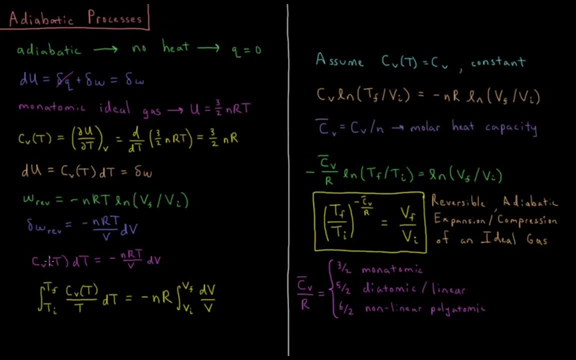 that's the amount of work that occurs during some very tiny change there. so we have constant volume. heat capacity times the change in temperature equals negative nRT over V times the change in volume. so we can integrate both sides here where we've got a DT over there and a DV over there. but first we're going to 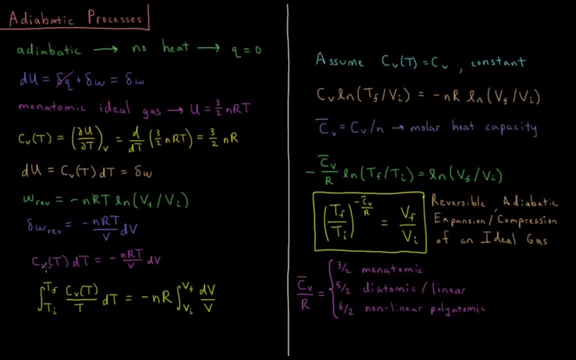 have to divide both sides by T so that we isolate the things that depend on temperature over here and the things that depend on volume over here. so we're doing some separation of variables here, a standard technique from an ordinary differential equations class. so we have the integral from the initial temperature. 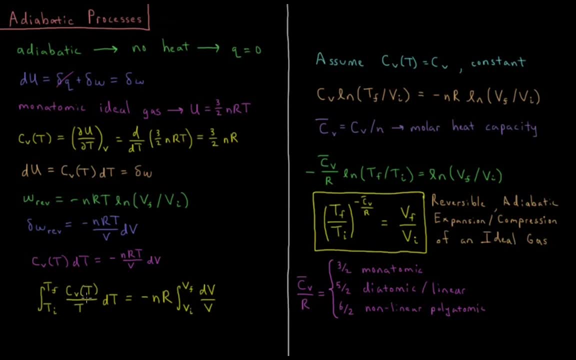 to the final temperature of the constant volume. heat capacity divided by temperature, integrated with respect to T equals, I can factor out negative nRT over nr. that doesn't depend on v equals negative number of moles times gas constant times the integral from the initial volume to the final volume of dv over v. All right, so if we assume 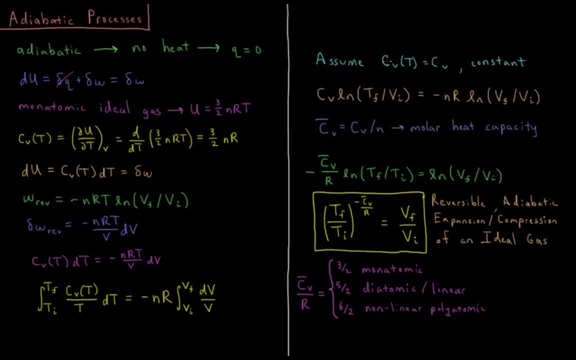 that during this change in temperature range that our constant volume heat capacity is approximately constant, which is usually a pretty good approximation. if this is a mild change in temperature, say if it's only a couple kelvin or tens of kelvin, it's probably a reasonable. 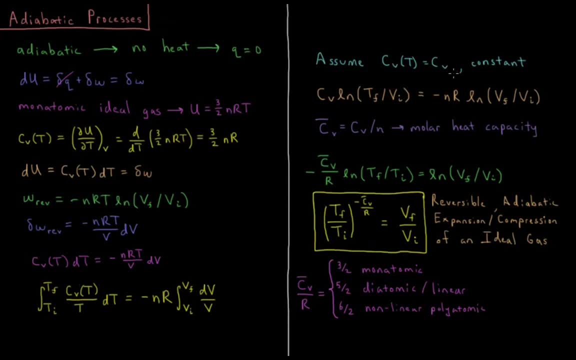 approximation. If it's hundreds of kelvin, it's probably not. So if we assume that this is a constant with respect to t, then what we get is cv log: t final over t initial equals negative nr. log v final over v initial, where we've done both of these integrals and evaluated at. 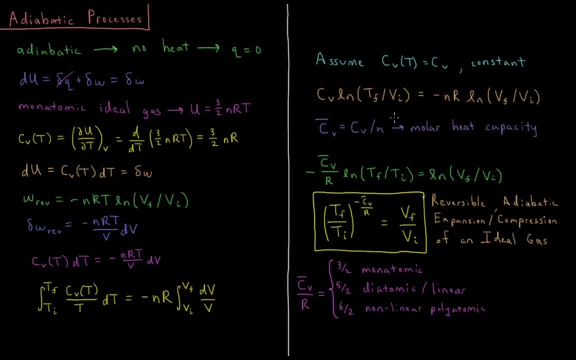 the initial and final conditions. So so we can also define a quantity now called the molar heat capacity. So the constant volume molar heat capacity, cv bar, is just the constant volume heat capacity divided by the number of moles, So the heat capacity per mole of particles typically, as any molar quantity will be. we just 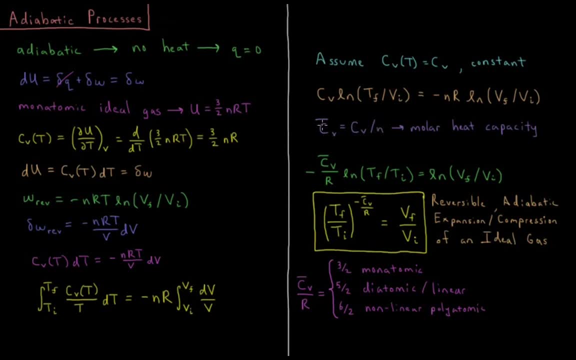 take whatever quantity we have, divide by n, and now put a bar on top. So I've divided out the n's here, so I can also divide both sides by r, and I can also divide both sides by r, and I can also. 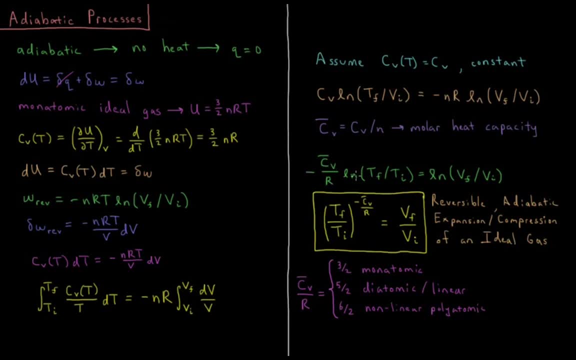 divide both sides by r and I get negative cv bar over r. log t final over t initial equals log v final over v initial. So now I can take both sides to the power of e and get rid of those natural logs. and what I get as a result? 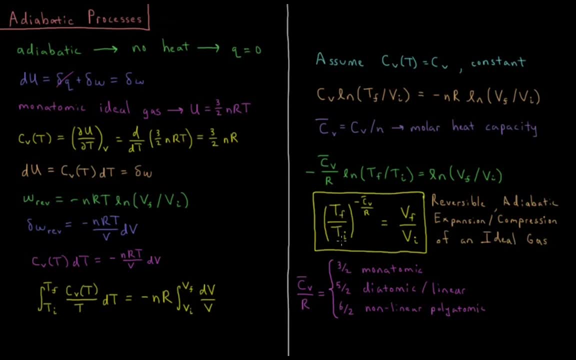 is that the quantity t final over t initial, taken to the power minus cv bar over r, equals v final over v initial. So this is my relationship between temperature and volume for the reversible adiabatic expansion or compression of an ideal gas. So the relationship here. note that in isothermal processes we had the temperature as a constant. 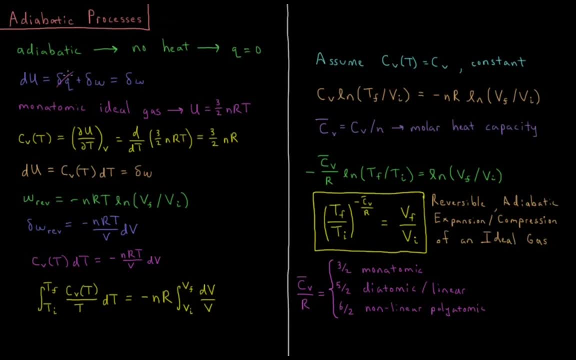 So the temperature was a constant and we added in whatever heat we needed to cancel out the work that we were doing Here. we have no heat, so that work isn't getting cancelled out. our energy is changing and thus our temperature is changing. 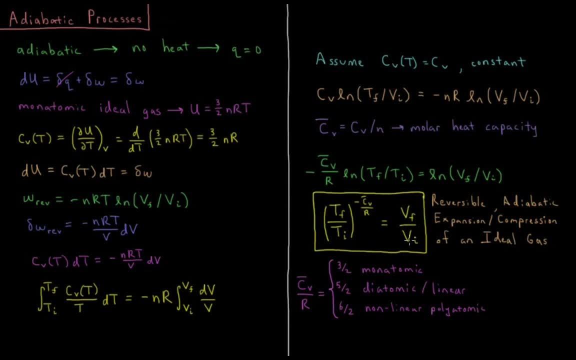 and that temperature change. we can tell from how the volume changes and what the heat capacity of our system is. So the molar heat capacity changes based off the type of gas that we have, the type of ideal gas that we have For monatomic ideal gases they only have translational motion. 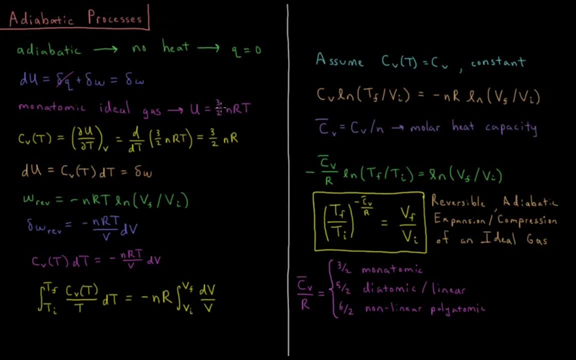 So from statistical mechanics we see that you get a one-half nRT from each kind of degree of freedom. So they have translation in x, y and z. Three of them, Or three-halves R for a monatomic gas. 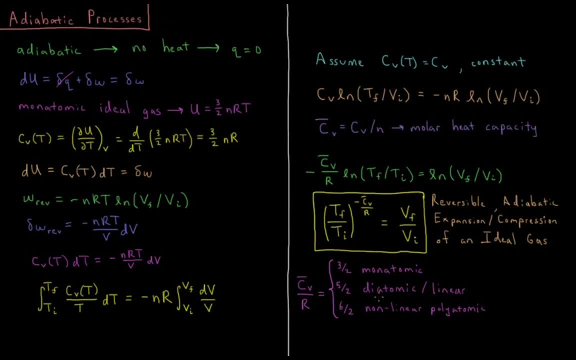 For diatomic or linear ideal gases, they have those three translations plus two rotations. So you get five-halves R for your heat capacity or your molar heat capacity. And for nonlinear polyatomic molecules you have three rotations and three translations. 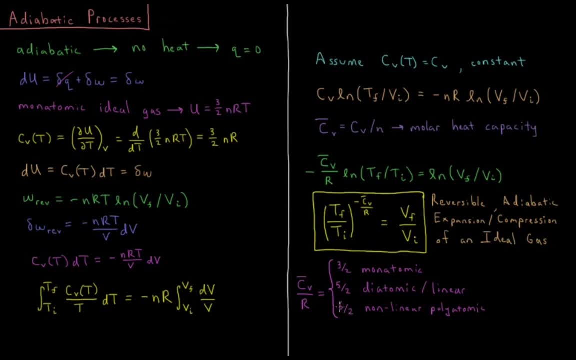 So your heat capacity is six-halves R or three R for your molar heat capacity. So when you're using this equation here, you need to know what are the initial and final volumes, what is the initial temperature, and paying attention to what kind of ideal gas you have. 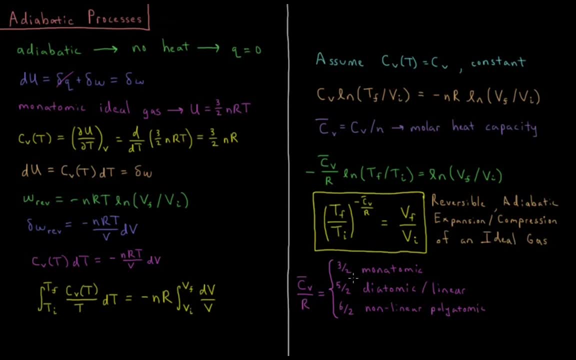 so you know what to substitute in for Cv-bar over R.